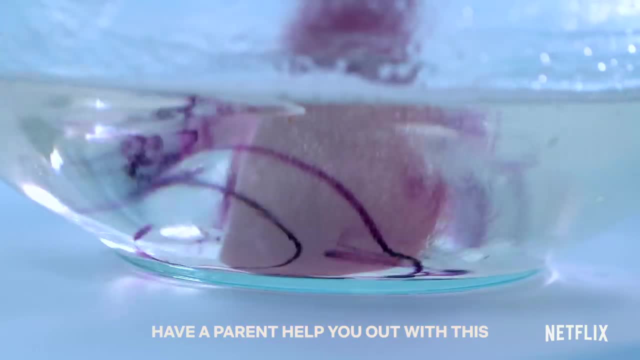 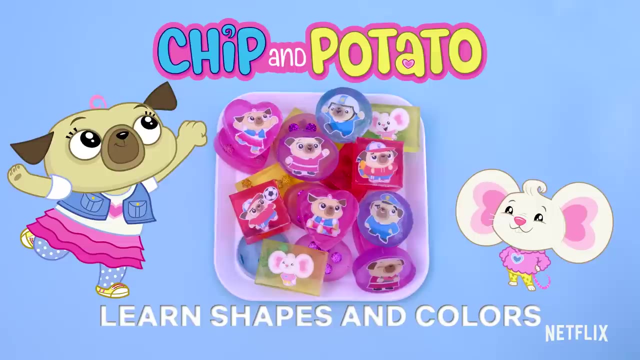 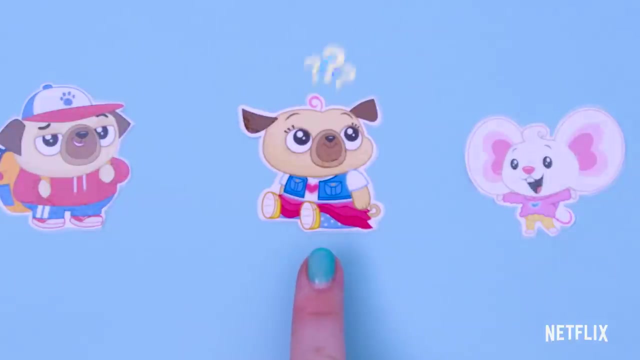 Have a parent help you out with this. Let's learn shapes and colors with Chip and Potato. Hi, I'm Chip and this is my potato. snuggly Do you see, Chip? What color is Chip's skirt? Pink, You got it. Chip's skirt is pink. 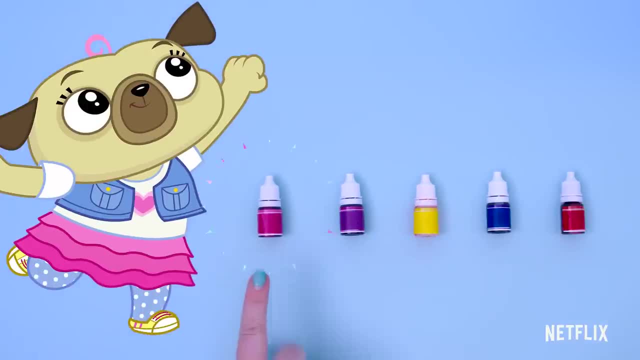 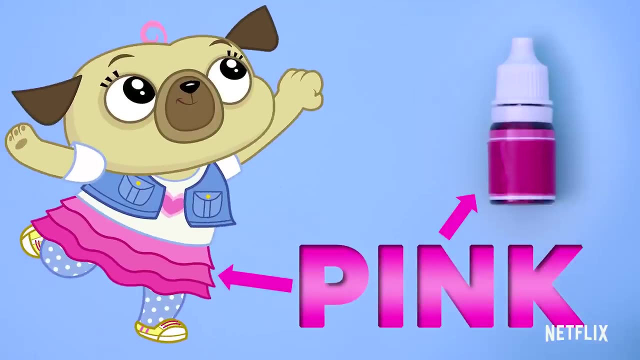 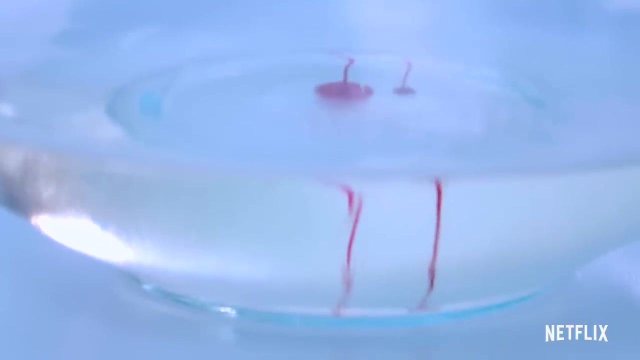 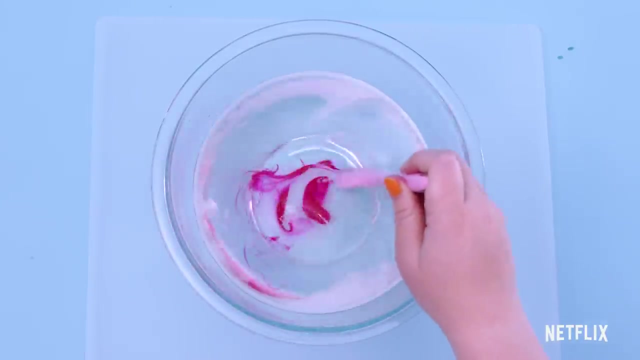 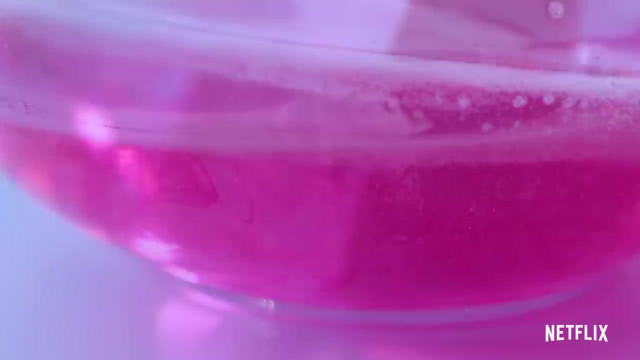 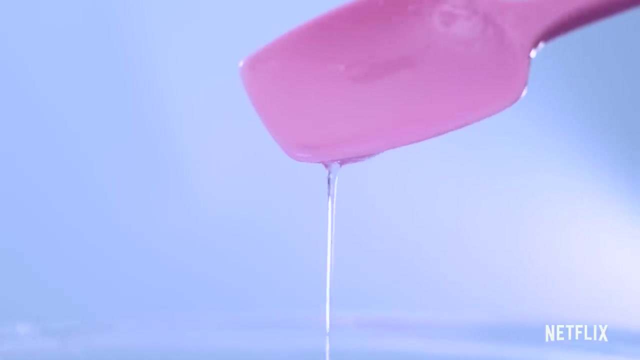 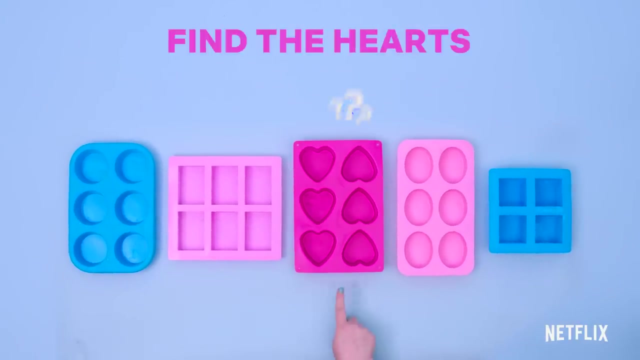 Which bottle is pink? Yes, you got it Pink, just like Chip's skirt. Chip's skirt is pink, and so is this bottle. Let's make pink soap that is shaped like a heart, Which one of these has hearts? That's right. Let's make soap shaped like hearts. 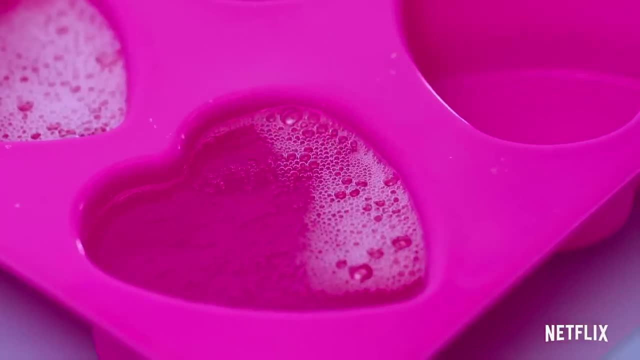 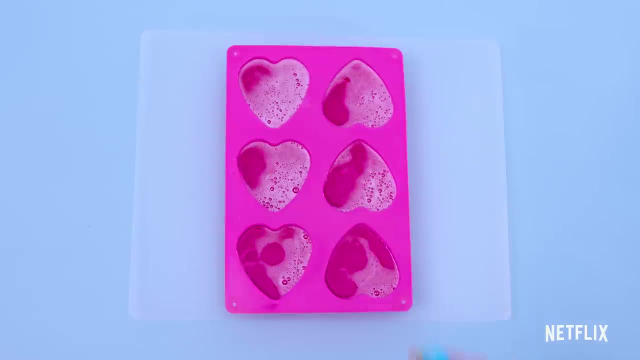 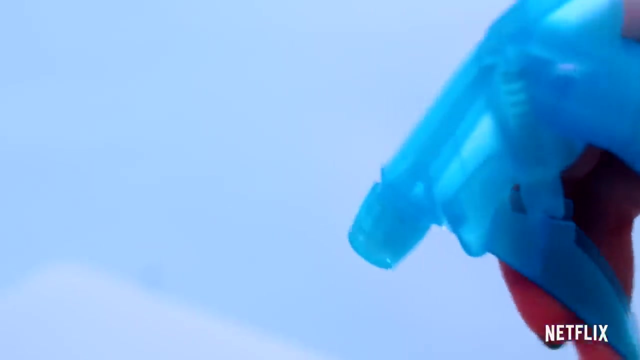 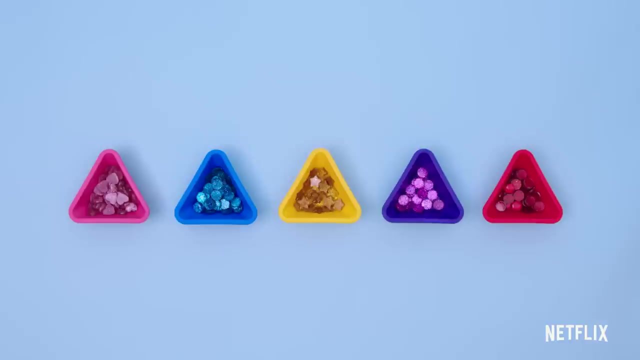 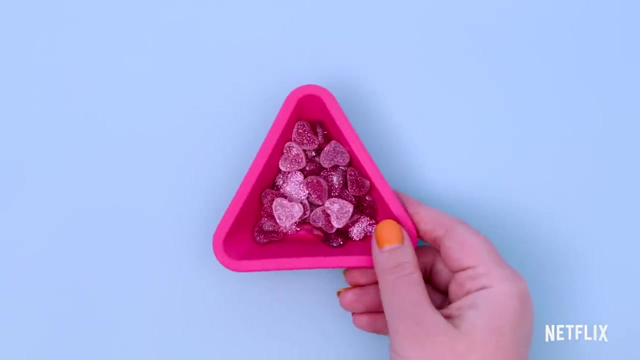 Which one of these bowls is pink? Is this one pink? No, that's blue. Is this one blue? Is this one pink? Nope, that's yellow. Is this one pink? Yes, There are pink gems in the pink bowl. 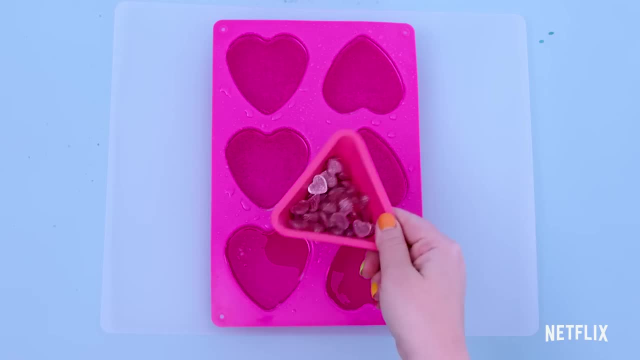 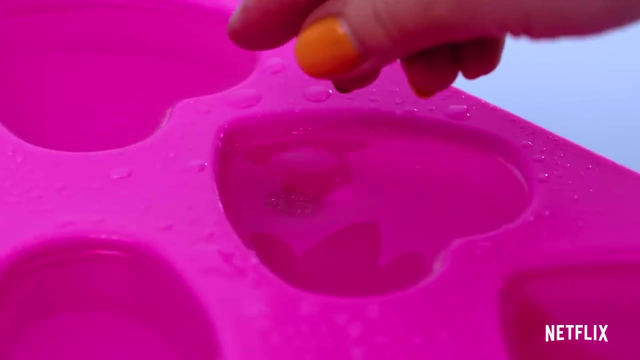 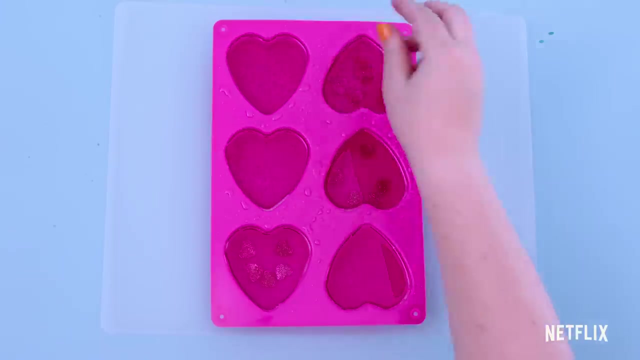 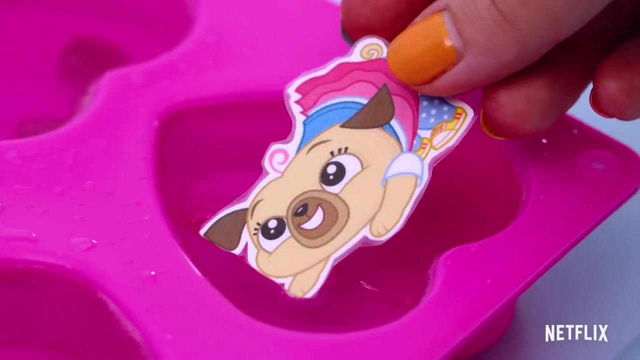 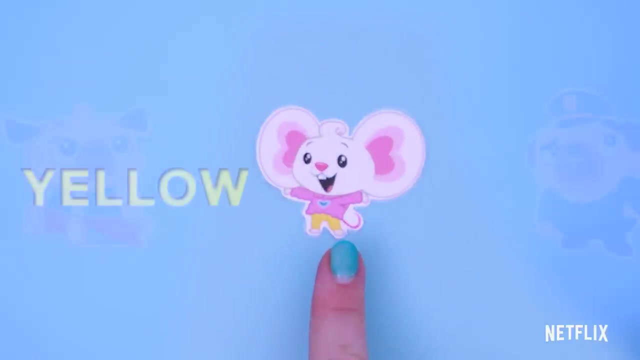 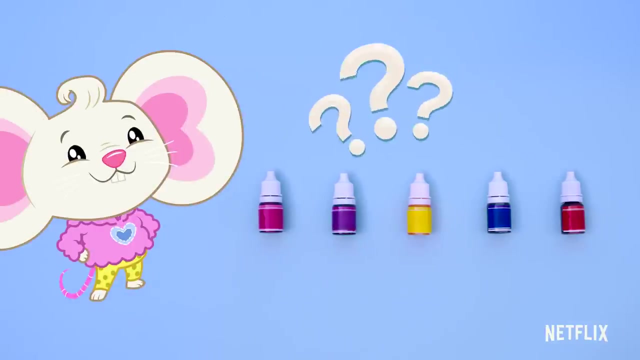 Let's add those to the pink soap. And last but not least, let's add Chip. Can't wait to wash my hands with my good friend Chip. Where's Potato? Let's find yellow with Potato. I love yellow. Which bottle is yellow? 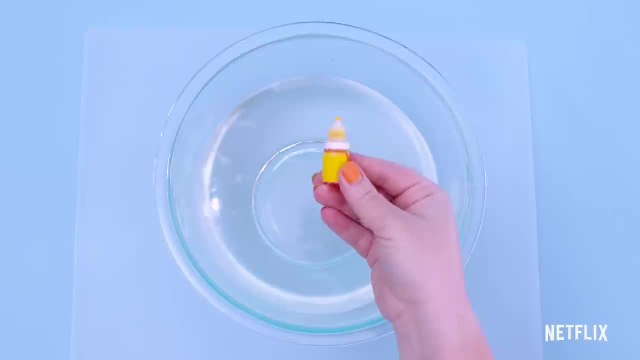 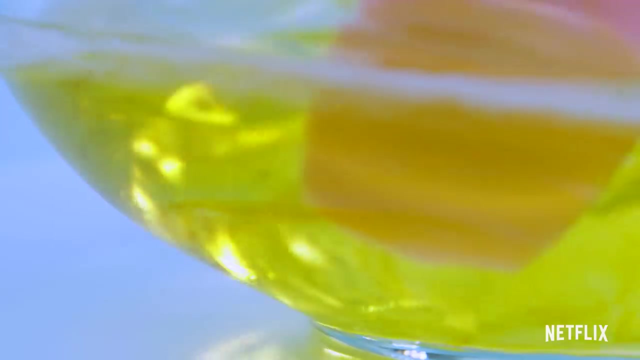 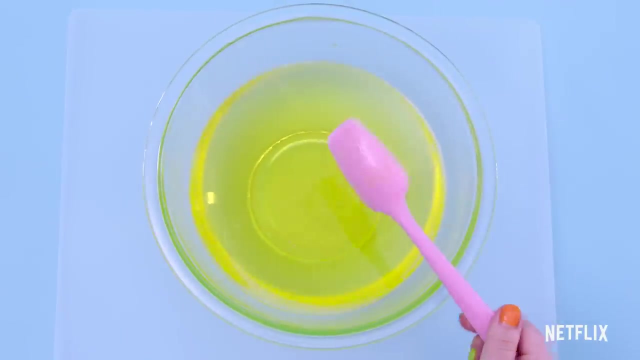 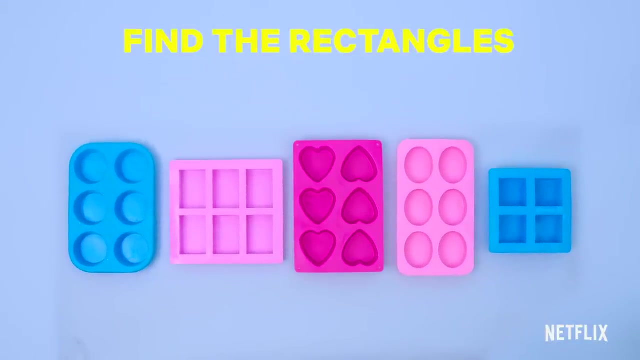 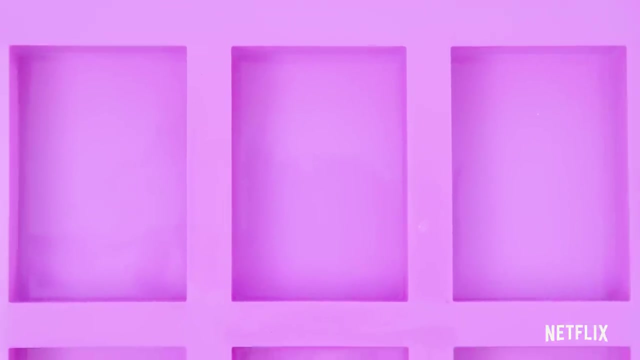 Yes, you got it Yellow. Let's make yellow soap that's shaped like a rectangle, Which one of these has rectangles? That's right. Rectangles have four sides: Two short ones, One, Two And two long ones, Three. 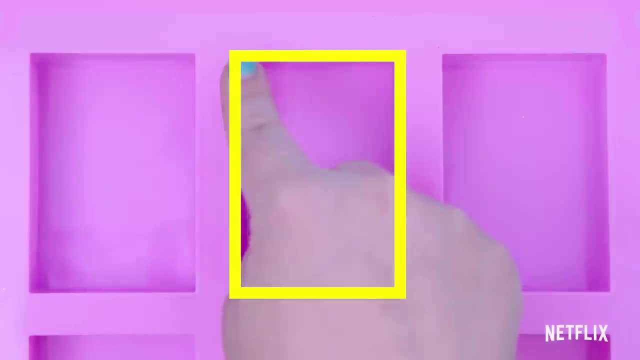 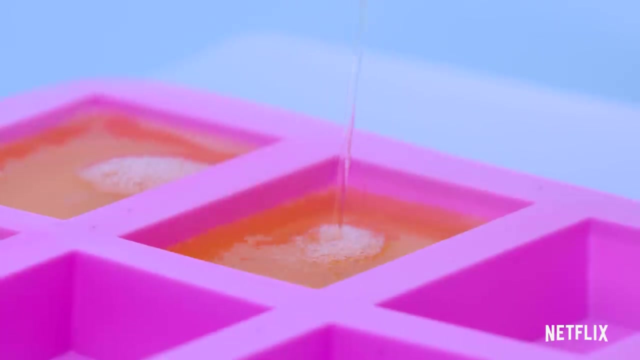 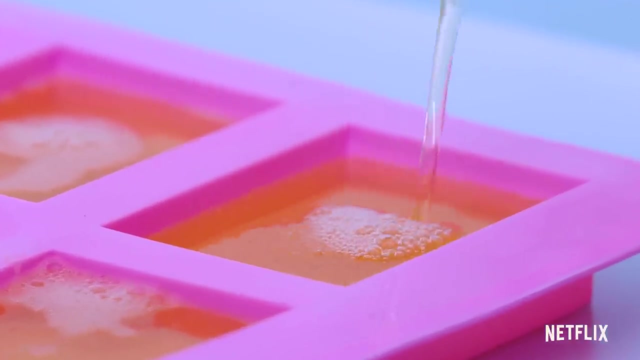 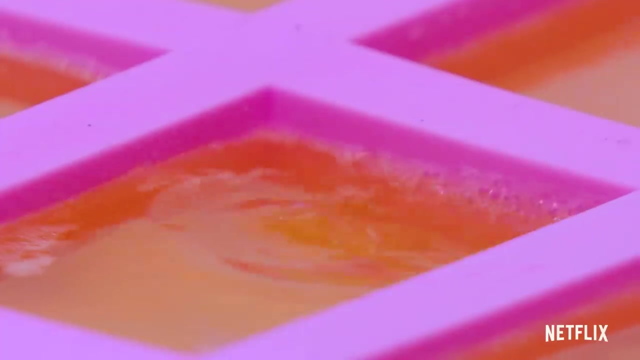 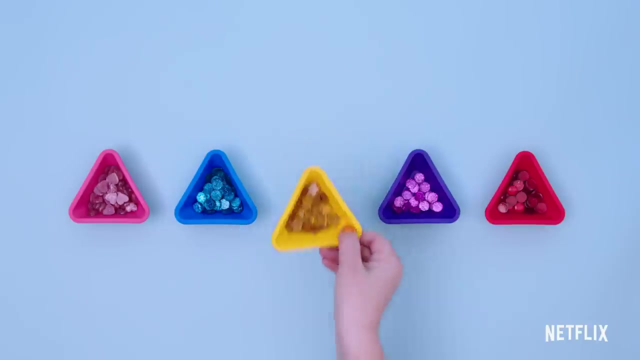 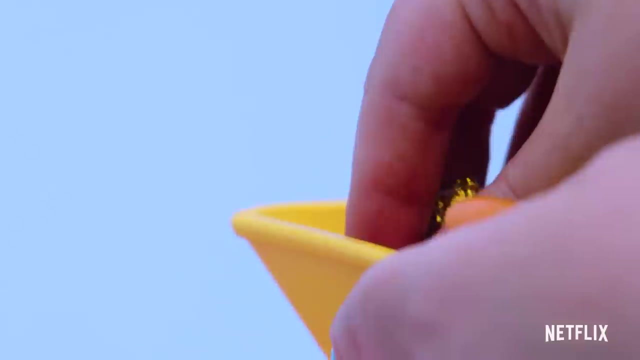 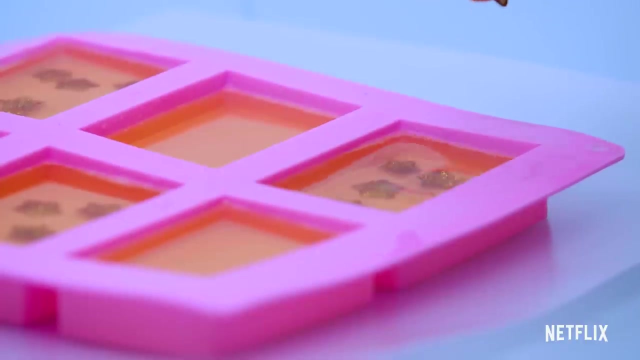 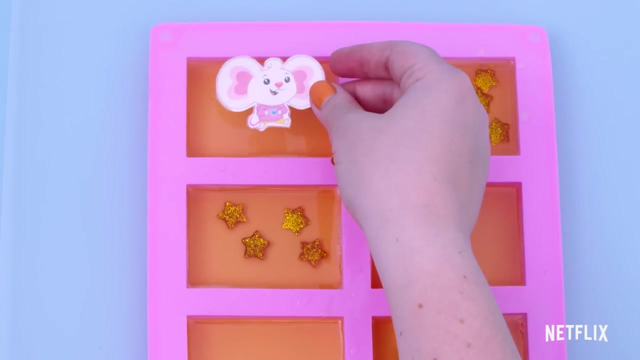 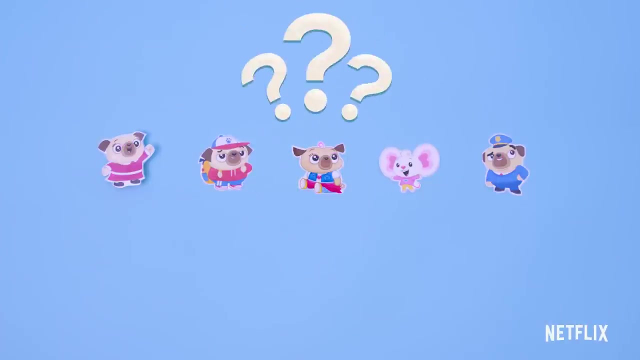 Four. Let's make rectangle soaps. which one of these bowls is yellow? yes, this bowl is yellow. there's yellow charms in the yellow bowl. let's add these to the yellow soap. and, last but not least, let's add potato. which character is wearing a red shirt? that's right, spud. 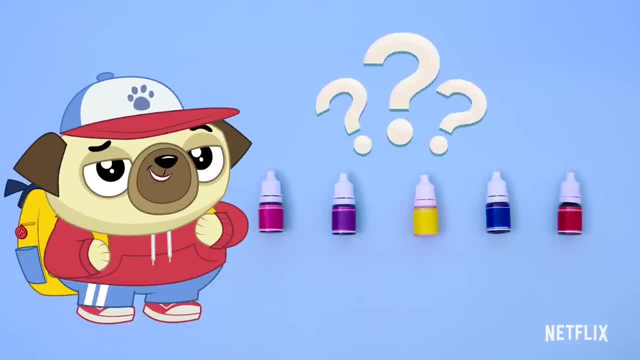 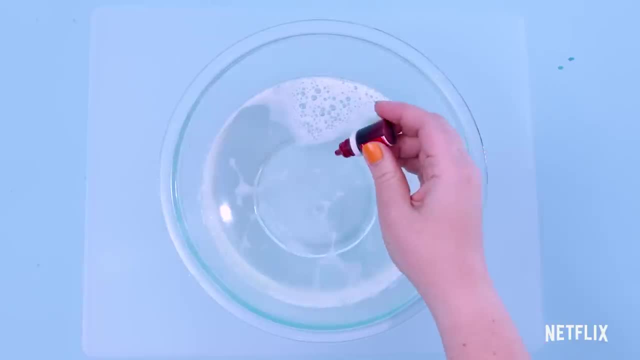 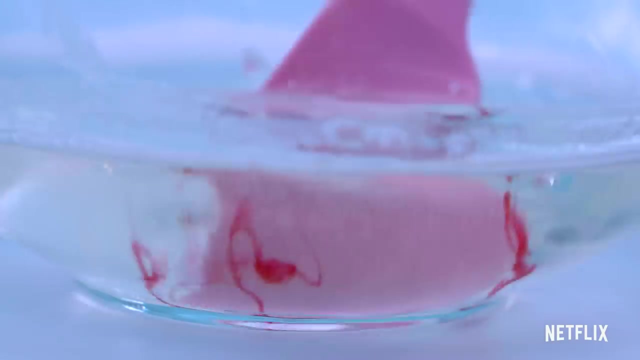 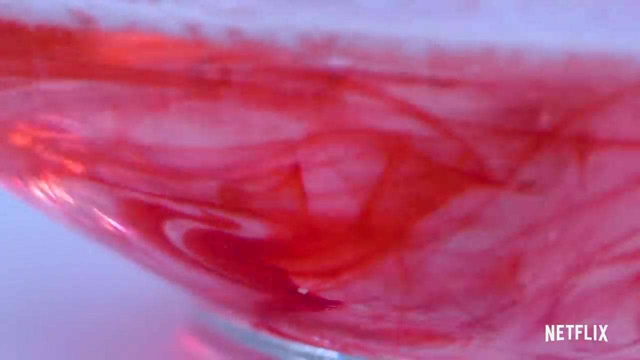 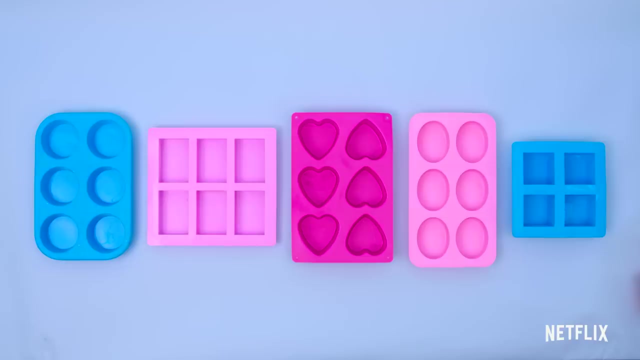 which character is wearing a red shirt? that's right. spud bottle is red- yes, you got it red. let's bottle is red. yes, you got it red. let's make this soap a square. make this soap a square. can you find the one with squares? that's. 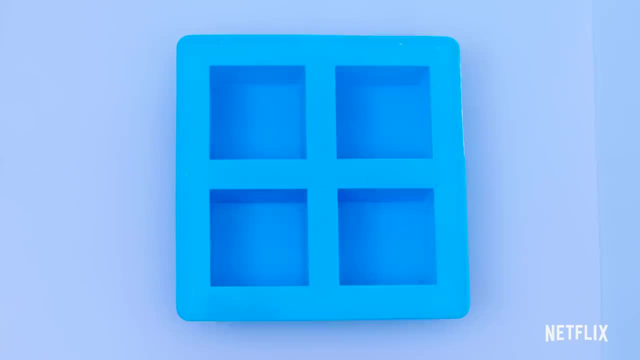 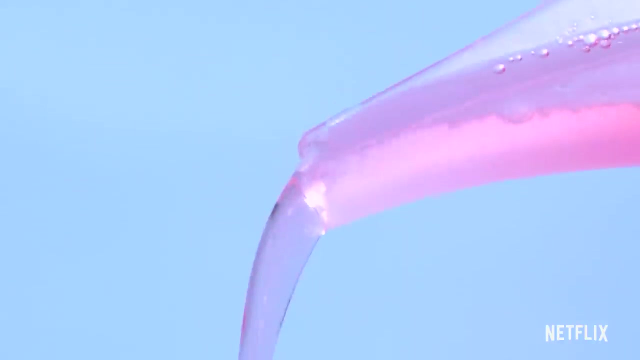 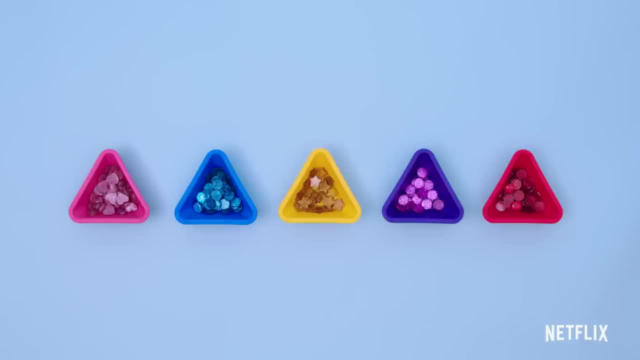 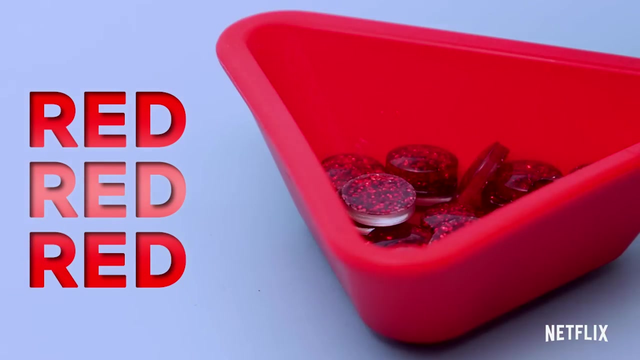 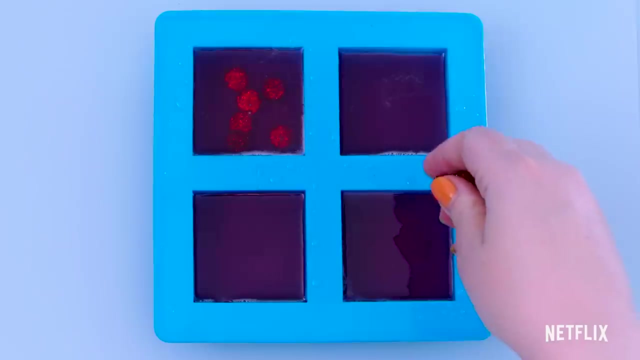 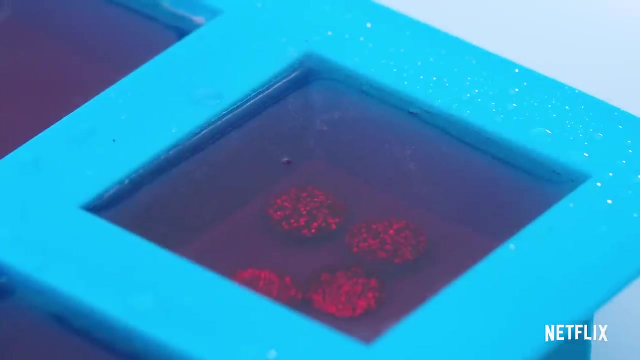 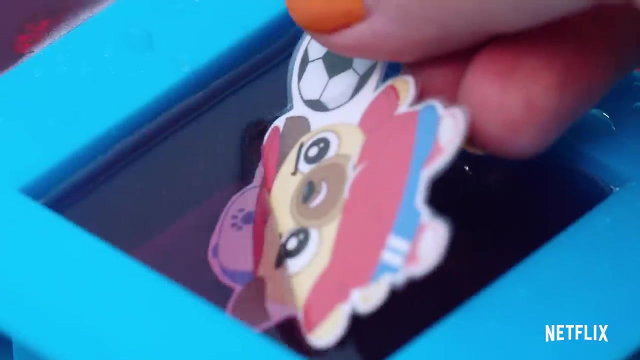 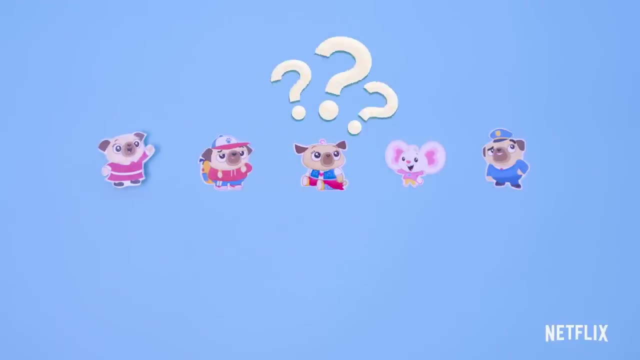 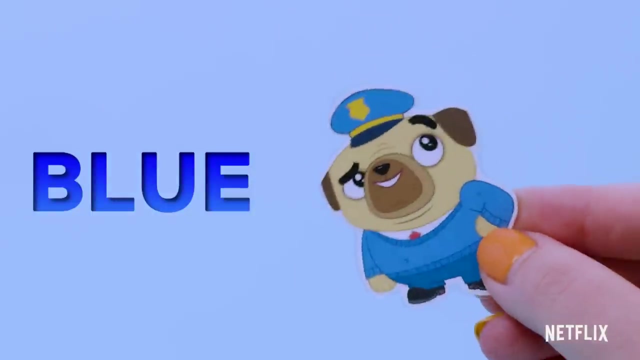 can't wait to wash my hands with spud. which character is wearing a blue hat and which character is wearing a blue hat? and which character is wearing a blue hat and blue clothes? Papa, Papa's outfit is blue blue clothes. Papa, Papa's outfit is blue blue clothes. Papa, Papa's outfit is blue huggy police to the rescue. which bottle? 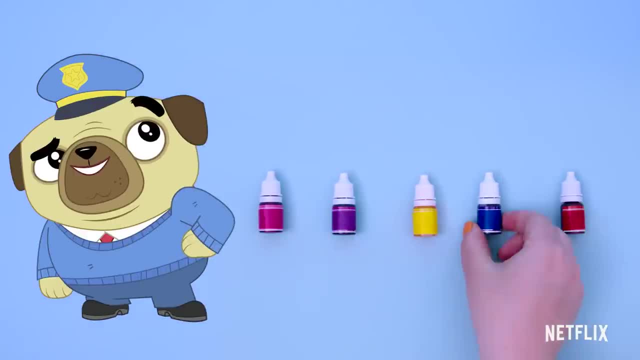 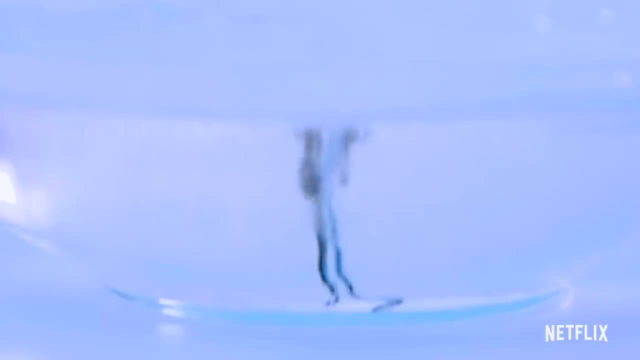 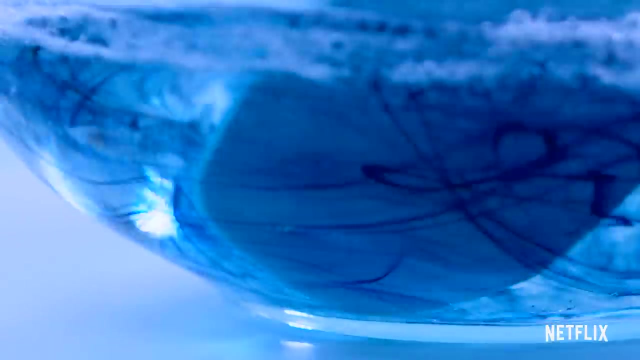 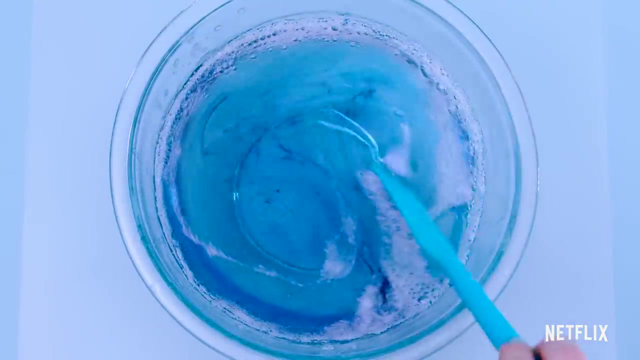 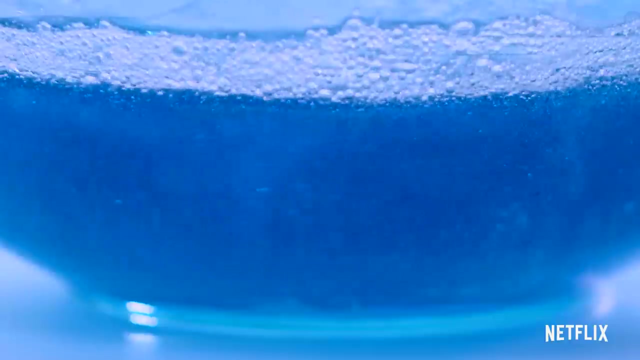 huggy police to the rescue. which bottle? huggy police to the rescue. which bottle is blue? yes, you got it blue, just like is blue. yes, you got it blue, just like is blue. yes, you got it blue, just like Papa's outfit. let's make blue soap that is shaped like. 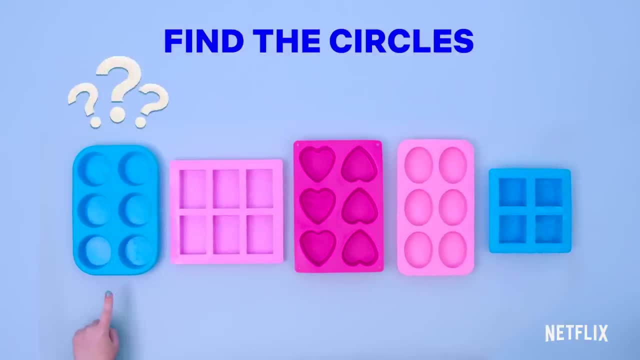 let's make blue soap that is shaped like. let's make blue soap that is shaped like a circle which one has circles. a circle which one has circles. a circle which one has circles. that's right. circles are round. let's. that's right, circles are round, let's. 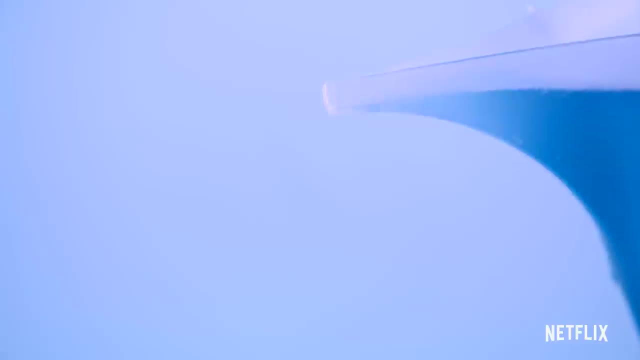 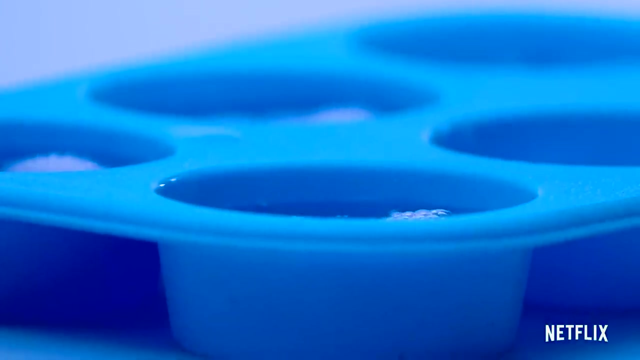 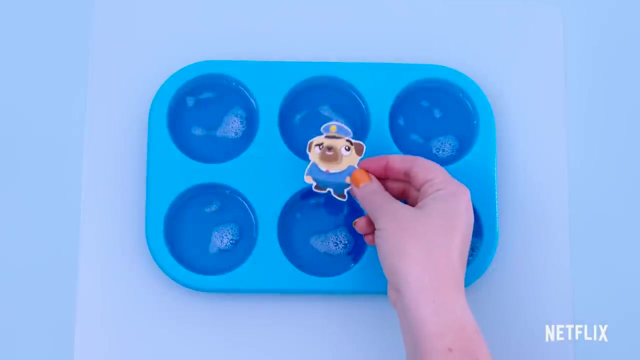 that's right. circles are round, let's make circle soaps. let's add Papa. Oh, make circle soaps. let's add Papa. Oh, make circle soaps. let's add Papa. Oh, Papa looks so cute in the blue soap. Papa looks so cute in the blue soap. 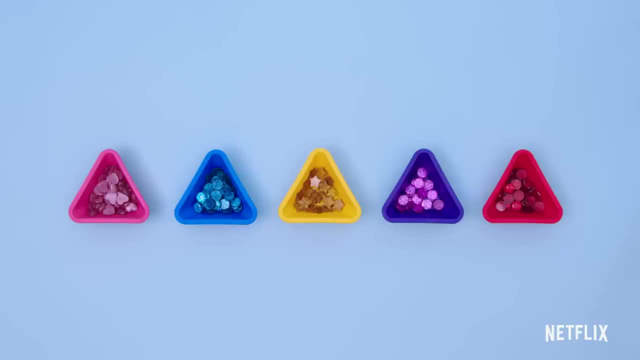 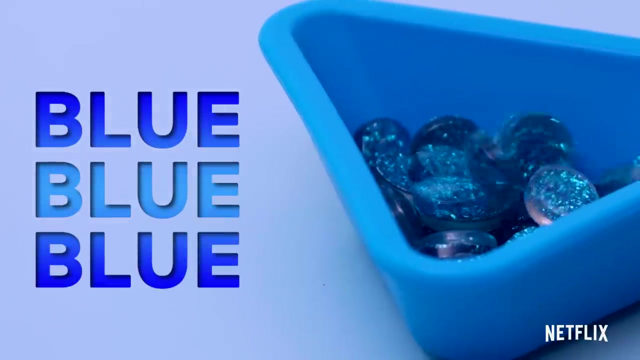 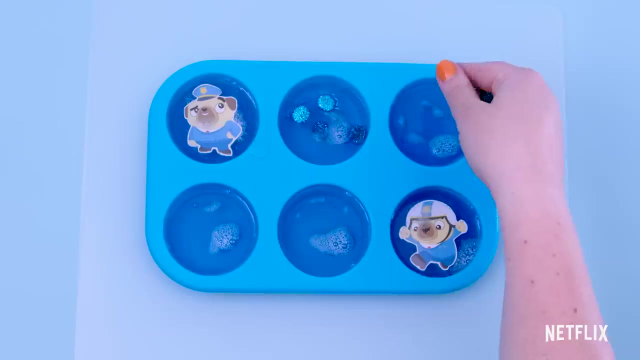 which one of these bowls is blue? is this one blue? no, that's red. is this one blue? nope, that's yellow. what about this one? yes, it's blue. there are blue gems in the blue bowl. let's add these to blue soap. I can't wait to wash my hands with Papa. can you find?